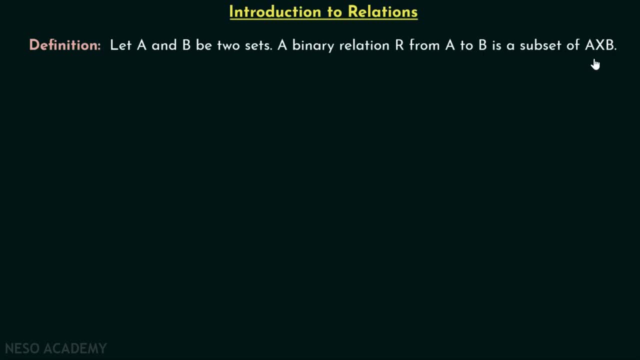 to B is a subset of A cross B. So a binary relation R from set A to set B is nothing but a subset of A cross B or Cartesian product of A and B. In other words we can say R is a subset of A cross B. Recall that A cross B is nothing but a set of all ordered pairs, A comma B, where 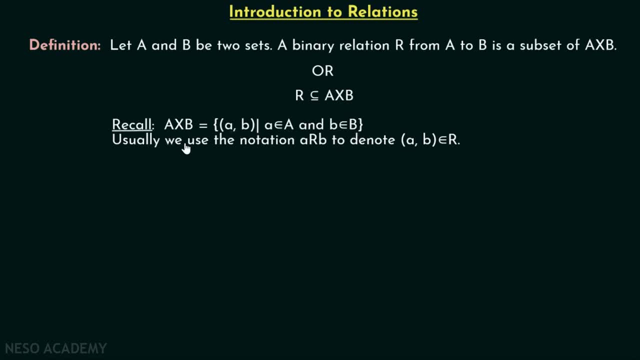 A belongs to set A and B belongs to set B. Usually we use the notation A R B to denote A comma. B belongs to R. Sometimes we call this A R B, as A related to B. A is not related to B is used to denote A comma. B does not belong to R. As simple as that. 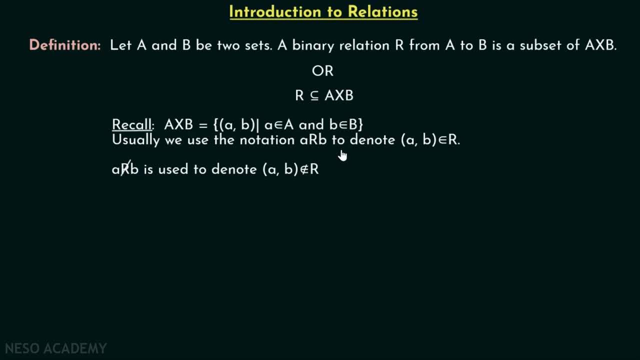 Right. So these are the notations we must remember. Apart from this, we must remember that R is a subset of A cross B, if R is defined from A to B. Now let's consider one example. Let's say A is a set which consists of 1,, 2,, 3 and B is a set which consists of these elements. 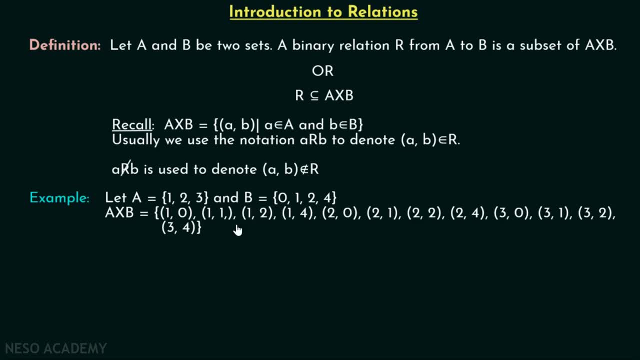 0, 1, 2, 4.. A cross, B must be this set which consists of all these ordered pairs, And in each ordered pair we have first element and second element, where the first element belongs to set B. Here you can clearly see we have these ordered pairs: 1, 0, 1, 1, 1, 2, 1, 4, 2,. 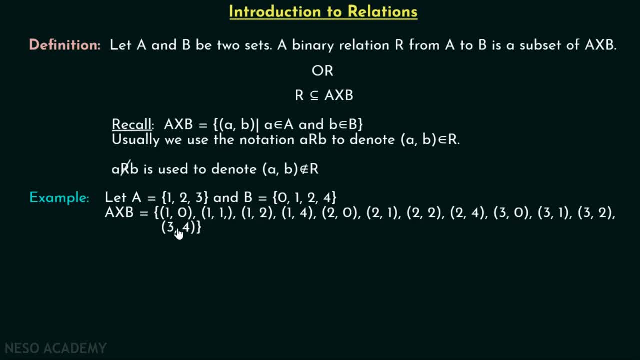 0, 2, 1, 2, 2, 2, 4, 3, 0, 3, 1, 3, 2, 3, 4.. Right, These are all the ordered pairs inside. 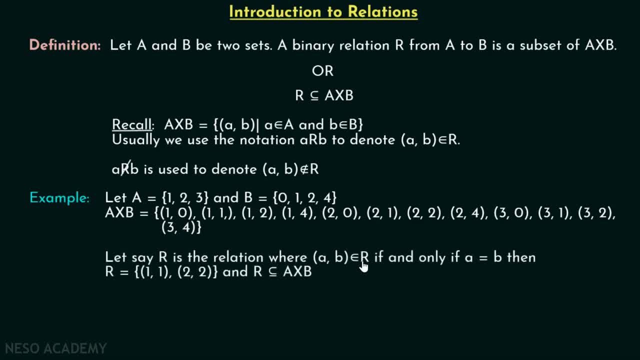 A cross B. Let's say R is the relation where A comma B belongs to R if, and only if, A is equal to B. I want to create this relation, R where A comma B, this ordered pair, belongs to R if, and only if, A is equal to B. 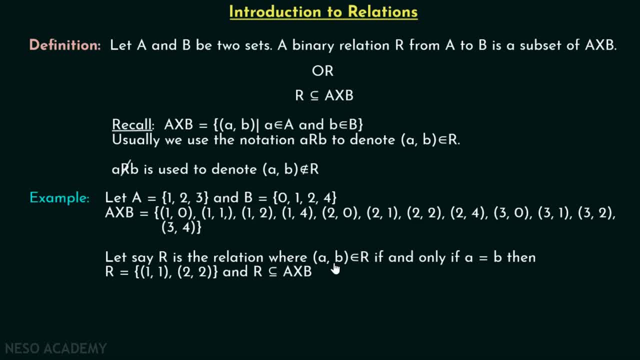 I want to include only those ordered pairs where A is equal to B. That means first element is equal to second element, Right? This is how R looks like. R is equal to this set, which consists of these ordered pairs: 1, 1 and 2, 2.. And you can clearly see this: R is a subset. 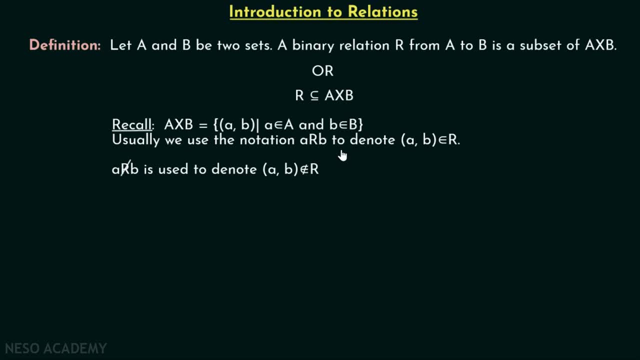 Right? So, these are the notations we must remember. Apart from this, we must remember that R is a subset of A cross B if R is defined from A to B. Now, let's consider one example. Let's say A is a set which consists of 1, 2, 3 and B is a set which consists of these elements 0, 1, 2, 4. A cross B must be this set which consists of all these ordered pairs. And in each ordered pair, we have first element and second element where the first element belongs to set B. Here, you can clearly see we have these ordered pairs 1, 0, 1, 1, 1, 2, 1, 4, 2, 0, 2, 1, 2, 2, 2, 4, 3, 0, 3, 1, 3, 2, 3, 4. Right? These are all the ordered pairs inside A cross B. Let's say R is the relation where A comma B belongs to R if and only if A is equal to B. I want to create this relation R where A comma B, this ordered pair belongs to R if and only if A is equal to B. 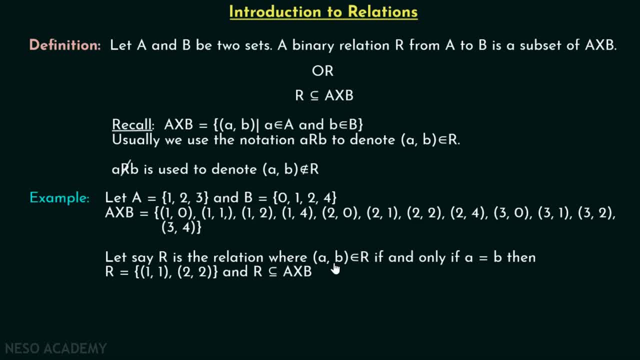 I want to include only those ordered pairs where A is equal to B. That means first element is equal to second element. Right? This is how R looks like. R is equal to this set which 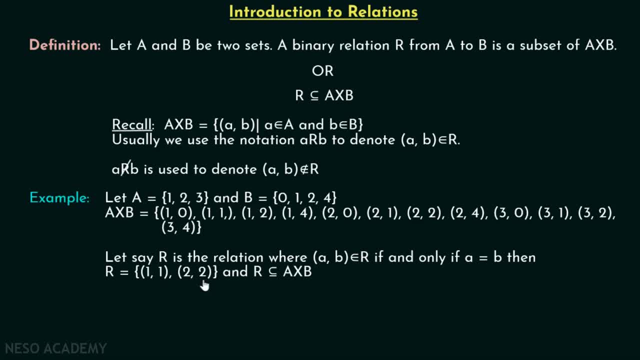 consists of these ordered pairs 1, 1 and 2, 2. And you can clearly see this R is a subset of A cross B because this R is derived from this A cross B. Isn't that so? 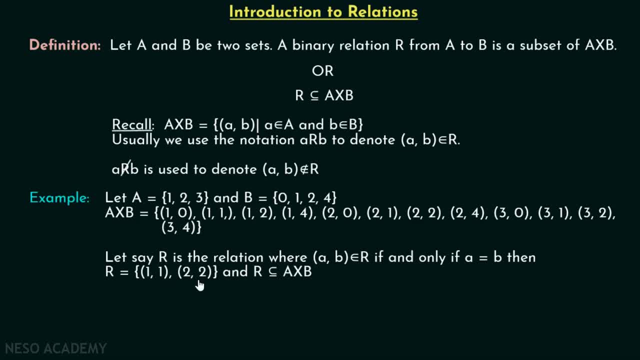 Now let's see the graphical representation of these ordered pairs. And this is how it looks like. 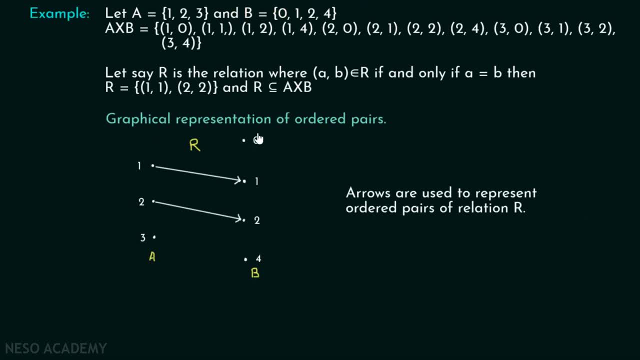 I have listed down all the elements of set A here and I have listed down all the elements of set B over here. We have 1, 2, 3 over here and 0, 1, 2, 4 over here. You can see I have drawn an arrow from this point to this point and from this point to this point. Actually 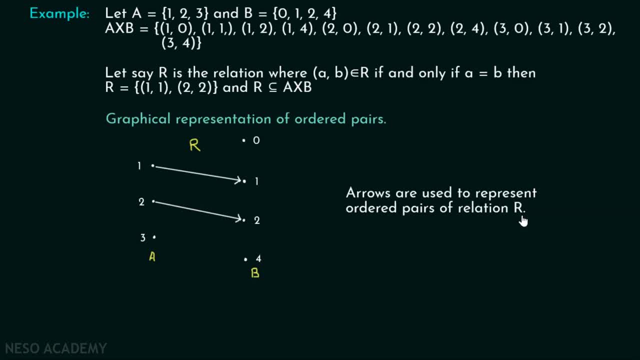 these arrows are used to represent ordered pairs of relation R. So this is nothing but relation R. Right? Here you can see this arrow is representing the ordered pair 1, 1 and this arrow is representing the ordered pair R. 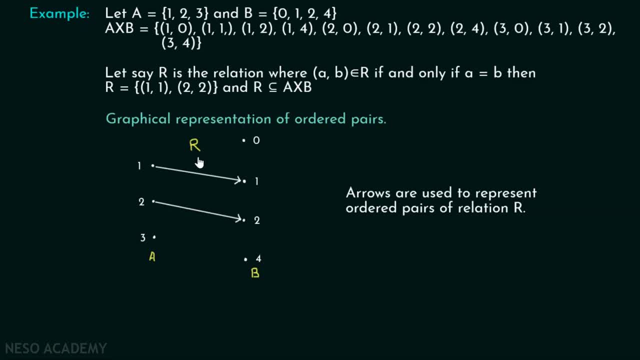 This whole mapping is relation R. Right? We have these ordered pairs 1, 1 and 2, 2. So this is the graphical representation of these ordered pairs and eventually this means we are talking about relation R. Right? We have seen how to define a relation from A to B. 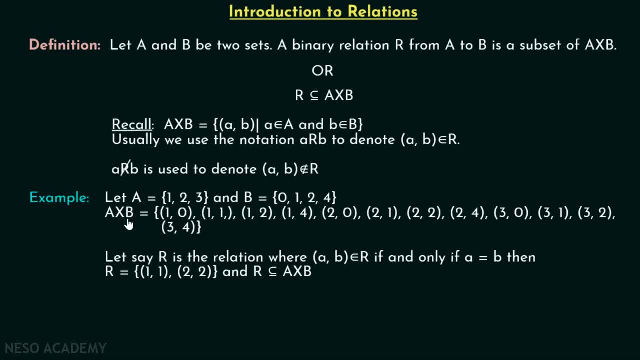 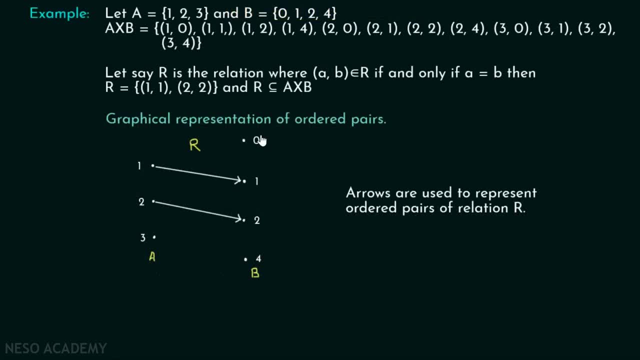 of A cross B, because this R is derived from this A cross B, Isn't that? so Now let's see the graphical representation of these ordered pairs, And this is how it looks like. I have listed down all the elements of set A here, and I have listed down all the elements. 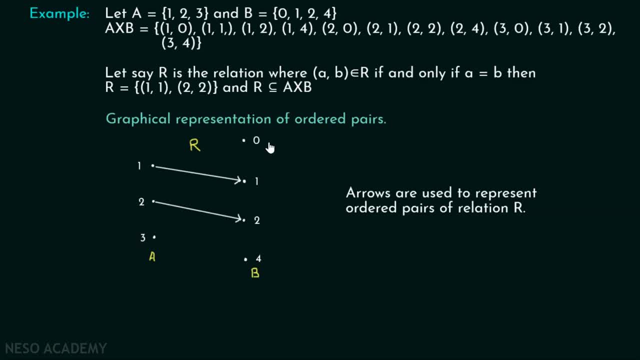 of set B over here. We have 1,, 2,, 3 over here and 0,, 1,, 2,, 4 over here. You can see, I have drawn an arrow from this point to this point and from this point to this point Actually. 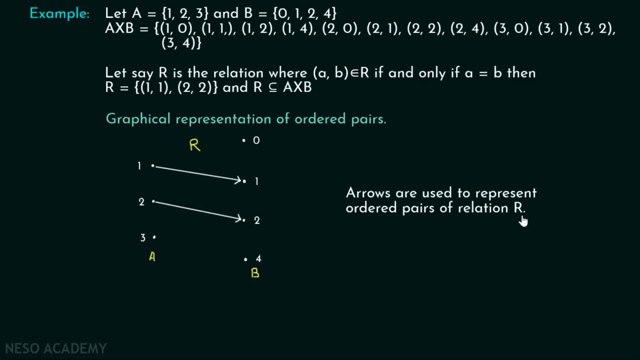 these arrows are used to represent ordered pairs of relation R. So this is nothing but relation R Right. Here you can see, this arrow is representing the ordered pair 1, 1 and this arrow is representing the ordered pair R. This whole mapping is relation R. Right. We have these ordered pairs 1, 1 and 2, 2.. So 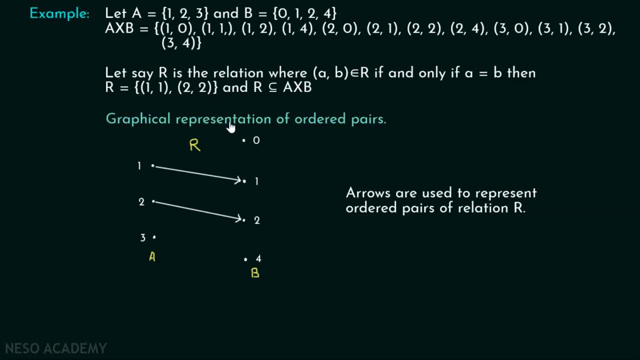 this is the graphical representation of these ordered pairs and eventually this means we are talking about relation R. Right, We have seen how to define a relation from A to B. Now we will see how to define a relation from a set to itself, A relation on a set. A is 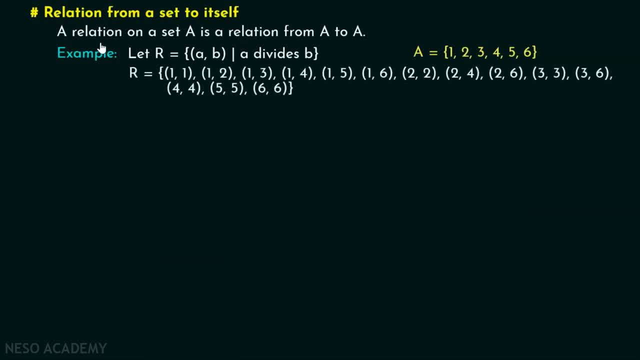 a relation from A to A. Please remember this: A relation on a set A is a relation from A to A. Let's consider one example. Let's say R is a set which consists of these ordered pairs: A, B. where A divides B, This relation is defined on set A, ie 1, 2, 3,, 4, 5, 6.. 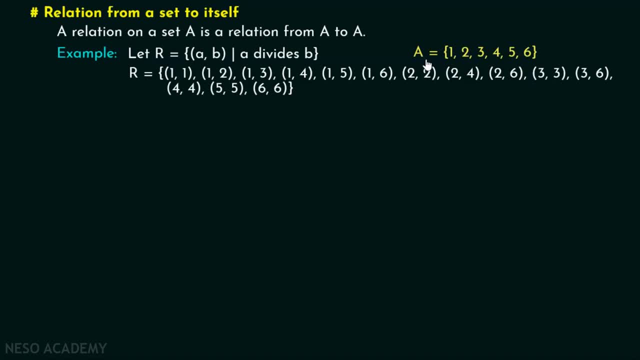 Obviously, we first have to take A cross, A ie Cartesian product of A with itself, And then we can choose all the ordered pairs where the first element divides the second element. Right Here you can see, this is the relation so formed where the first element 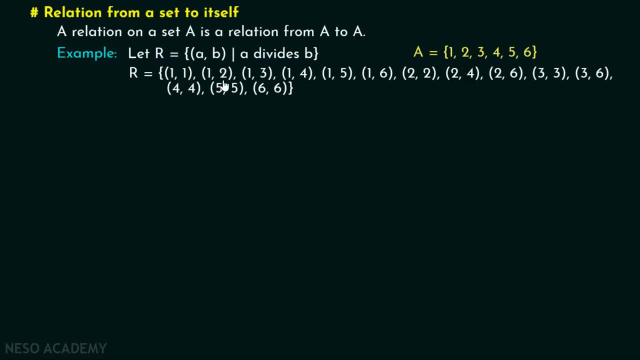 second element. You can clearly see that 1 divides 1, 1 divides 2, 1 divides 3, 1 divides 4, 1 divides 5, 1 divides 6, 2 divides 2, 2 divides 4, 2 divides 6, 3 divides 3, 3 divides 6, 4 divides 4, 5 divides. 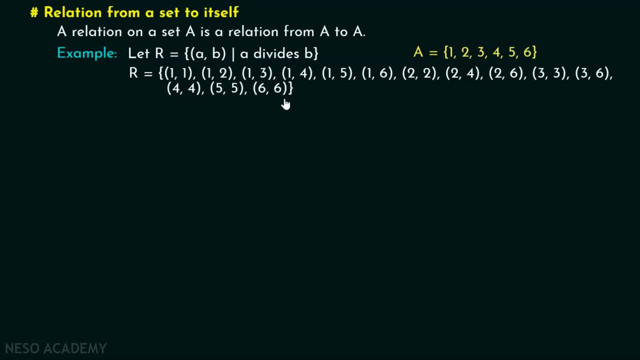 5, 6 divides 6.. These ordered pairs are included in R because first element in each ordered pair divides second element in that ordered pair, right. So this is our relation R and you can see this is a subset of A cross, A right, And this is the graphical representation of relation R. You can 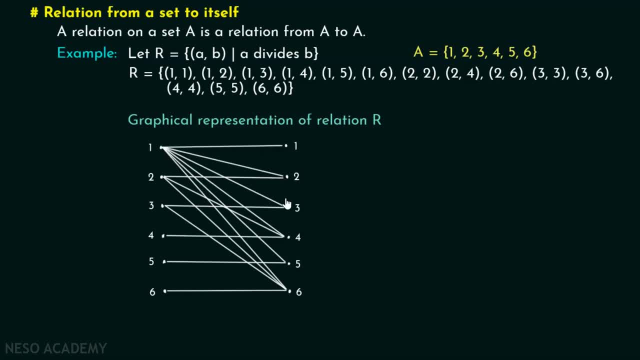 see these mappings right: From 1 to 1,, 1 to 2, 1 to 3, 1 to 4, 1 to 5, 1 to 6, then we have a mapping from 2 to 2, then 2 to 4, then 2 to 6, then we have a mapping from 3 to 3 and 3 to 6, then 4 to 4,. 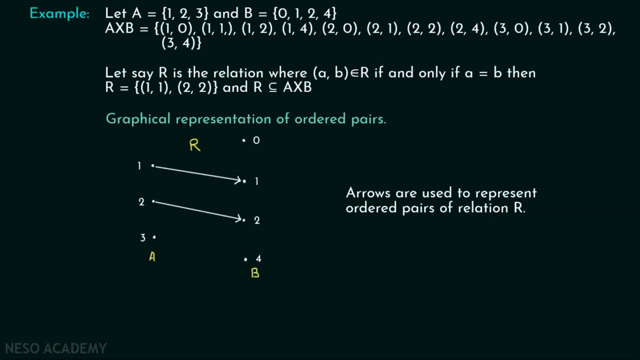 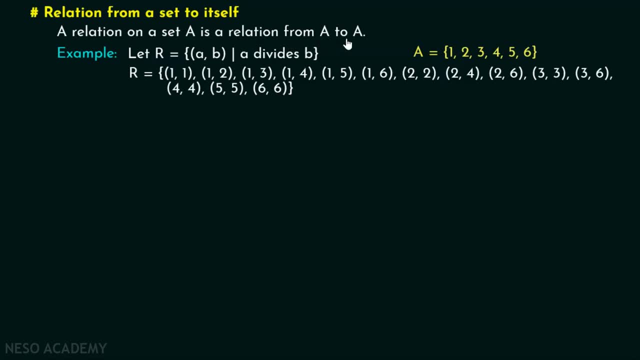 Now we will see how to define a relation from a set to itself. A relation on a set A is a relation from A to A. Please remember this. A relation on a set A is a relation from A to A. copy copy copy 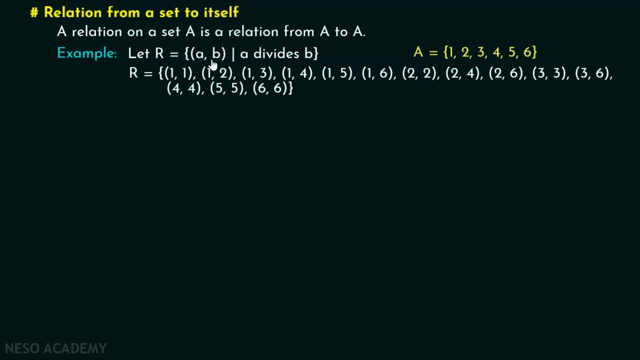 Let's consider one example. Let's say R is a set which consists of these ordered pairs where A divides B. This relation is defined on set A that is 1,2,3,4,5,6. Obviously we first have to take A cross A. That is Cartesian product of A with itself and then we can choose all the ordered pairs where the first element divides the second element. Right? Here you can see this is the relation SO formed where the first elements divide B. Right? 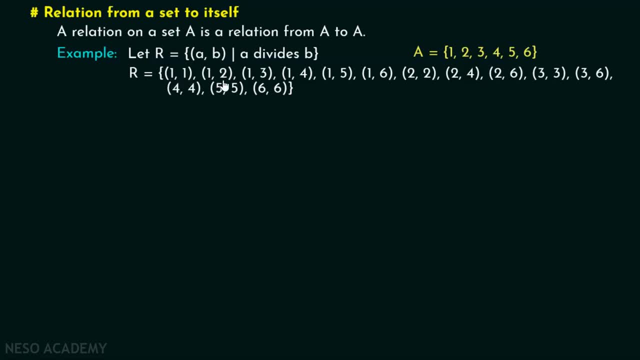 second element. You can clearly see that 1 divides 1, 1 divides 2, 1 divides 3, 1 divides 4, 1 divides 5, 1 divides 6, 2 divides 2, 2 divides 4, 2 divides 6, 3 divides 3, 3 divides 6, 4 divides 4, 5 divides 5, 6 divides 6. These ordered pairs are included in R because first element in each ordered pair 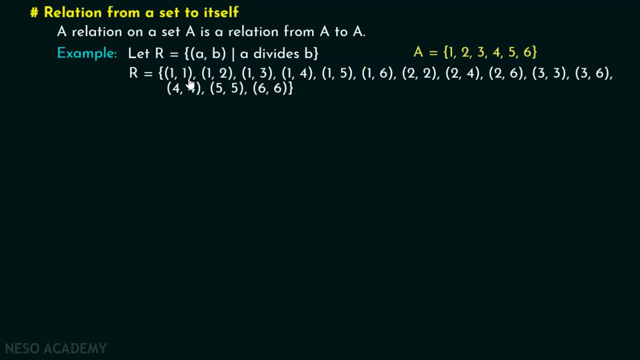 divides second element in that ordered pair, right? So, this is our relation R and you can see this is a subset of A cross A, right? And this is the graphical representation of relation R. You can see these mappings, right? From 1 to 1, 1 to 2, 1 to 3, 1 to 4, 1 to 5, 1 to 6. Then we have a mapping from 2 to 2, then 2 to 4, then 2 to 6. Then we have a mapping from 3 to 3 and 3 to 6, then 4 to 4, 5 to 5, 6 to 6. So, this is nothing but relation R, right? Now, after understanding how to define a relation from a set of elements, we can see that R is a subset of A cross A, right? And this is 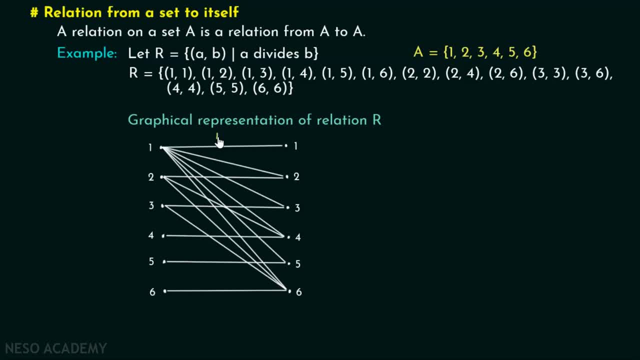 5 to 5,, 6 to 6.. So this is nothing but relation R. right Now, after understanding how to define a relation from a set of elements, we can see that R is a subset of A cross, A right, And this is. 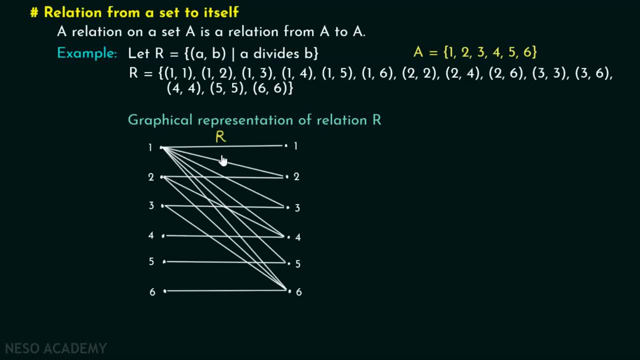 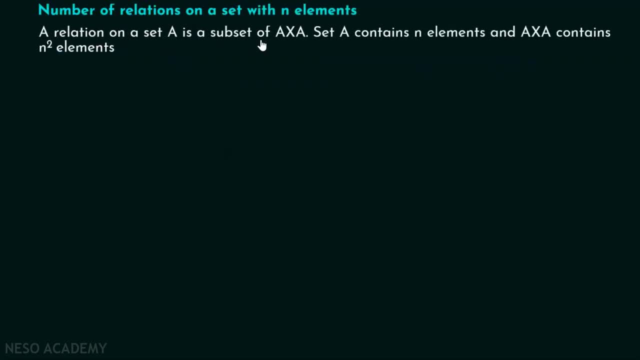 a set to itself. We will try to find out the number of relations on a set, that is, on a single set with n elements. okay, We know that a relation on a set A is a subset of A cross A. Let us suppose that set A contains n elements and A cross A contains n square elements. right, If it is the. 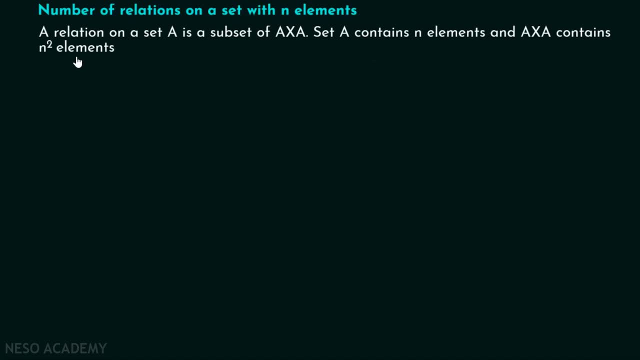 case that n elements are there in set A, then n square elements must be there in A cross A. We are interested in listing down all the subsets of A cross A means we are interested in listing down all the subsets of A cross A because we want to find out the number of relations on a set with n. 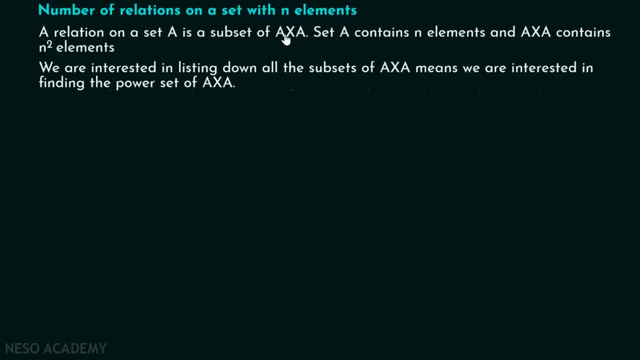 elements. We know that a relation on a set A is a subset of A cross A. that is why we are interested in finding all the subsets of A cross A right Means we are interested in finding the power set of A cross A. We know that P A is the power set of A and let us say A has n elements, then P A must. 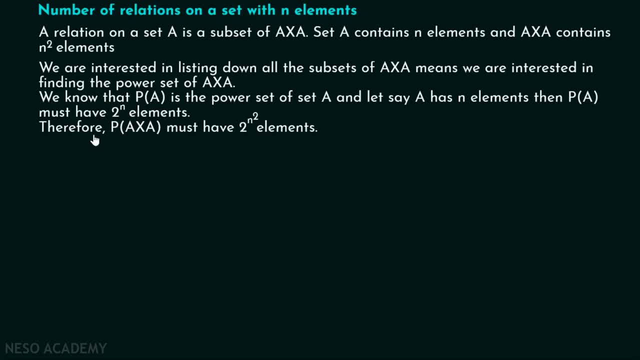 have 2 to the power n elements, Isn't that so? Therefore, P A cross A must have 2 to the power n square elements. right, P A cross A, that is, power set of A cross A, must have 2 to the power n square. 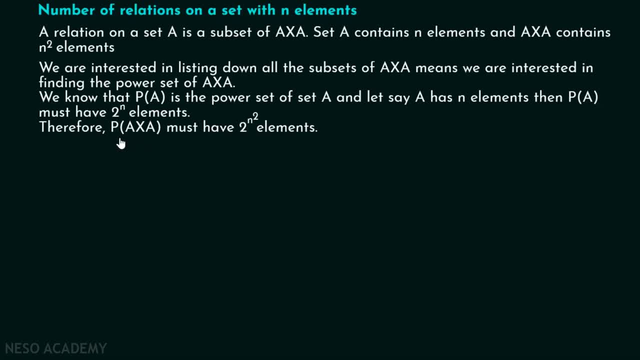 elements. because there are n square elements in A cross A, Then power set of A cross A must have 2 to the power n square elements. Hence the number of relations on a set A with n elements is equal to 2 to the power n square, which is actually the cardinality of P A cross A. 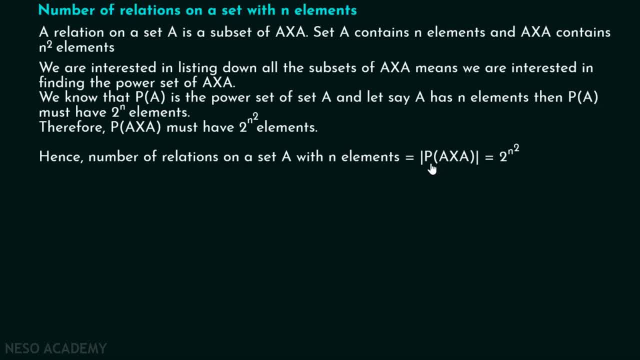 that is power set of A cross A. So the number of elements in power set of A cross A is actually equal to the number of relations on a set A Right. We know that cardinality of power set of A cross A is nothing but two to the power n square. 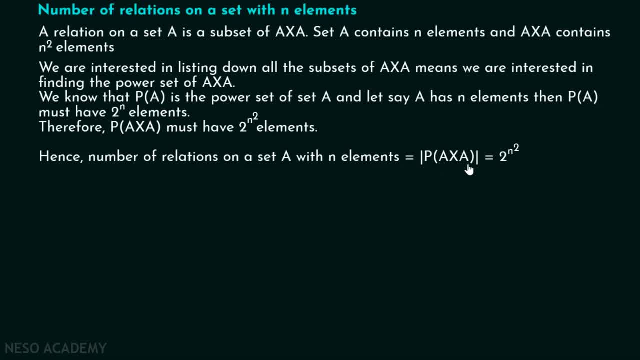 which represents the number of subsets of A cross. A Number of subsets means number of relations. Right Up to now, we have understood what is a relation. We have seen how to define a relation from a set A to set B. Then we have also seen how to define a relation. 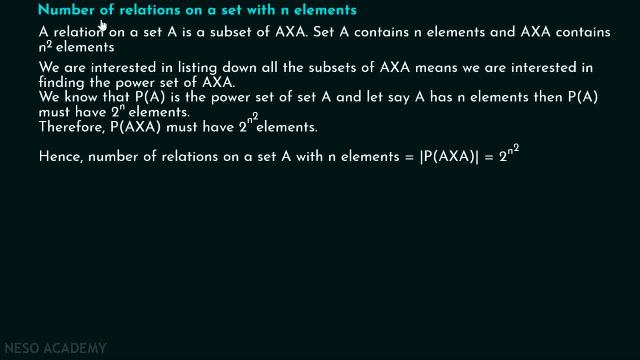 from a set to itself. Also, here we have seen how to find the number of relations on a set with n elements Right. We have seen this: that the number of relations on a set A with n elements is nothing but two to the power n square. 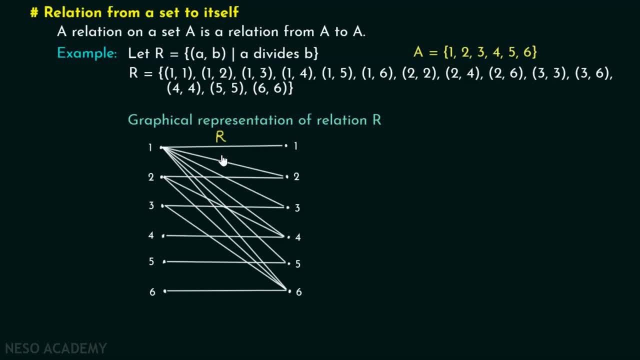 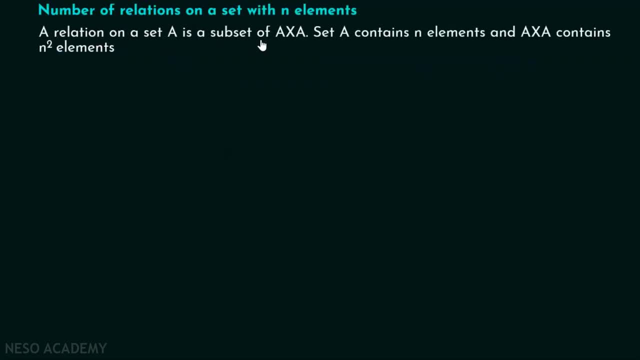 set with n elements, okay? We know that a relation on a set A is a subset of A cross A. Let us suppose that set A contains n elements and A cross A contains n square elements, right? If it is the case that n elements are there in set A, then n square elements must be there in A cross A. We are interested in listing down all the subsets of A cross A, means we are interested in listing down all the subsets of A cross A, because we want to find out the number of relations on a set with n elements. We know that a relation on a set A is a subset of A cross A, that is why we are interested in finding all the subsets of A cross A, right? Means we are interested in finding the power set of A cross A. We know that P A is the power set of A and let us say A has n elements, then P A must 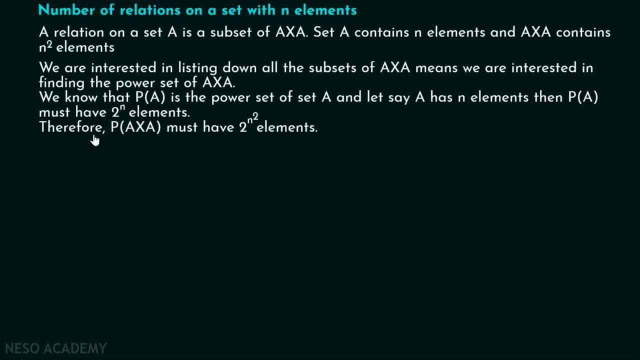 have 2 to the power n elements. Isn't that so? Therefore, P A cross A must have 2 to the power n square elements, right? P A cross A, that is power set of A cross A must have 2 to the power n square elements, because there are n square elements in A cross A. Then power set of A cross A must have 2 to the power n square elements. Hence, the number of relations on a set A with n elements is equal to 2 to the power n square, which is actually the cardinality of P A cross A. 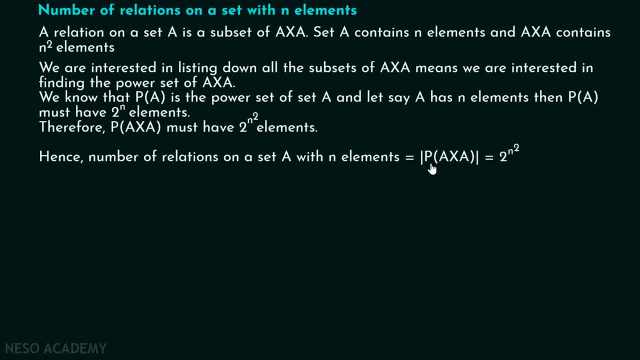 that is power set of A cross A. So the number of elements in power set of A cross A is actually equal to the number of relations on a set A. Right? We know that cardinality of power set of A cross A is nothing but two to the power n square, which represents the number of subsets of A cross A. 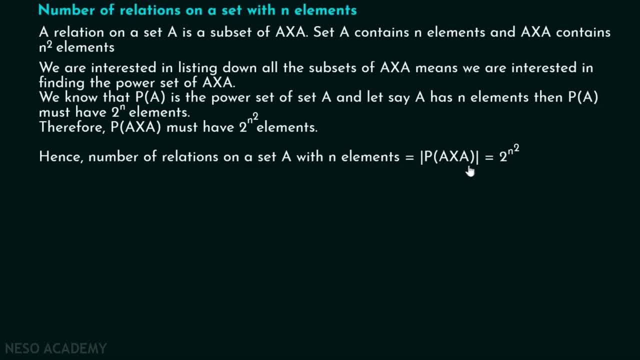 Number of subsets means number of relations. Right? 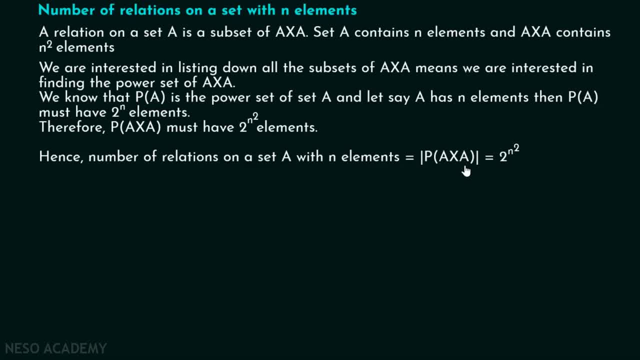 Up to now we have understood what is a relation. We have seen how to define a relation from a set A to set B. Then we have also seen how to define a relation from a set to itself. Also, here we have seen how to find the number of relations on a set with n elements. 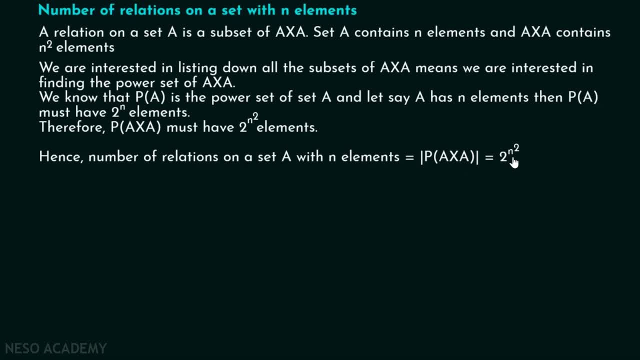 Because we know that in set A cross A we have n square elements and the power set of A cross A has two to the power n square elements. Right In the next presentation we will discuss types of relations. Okay, friends, this is it for now. Thank you for watching this presentation. 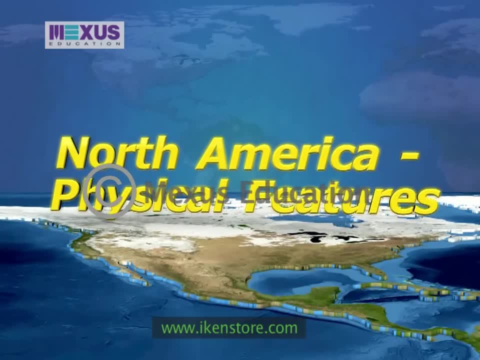 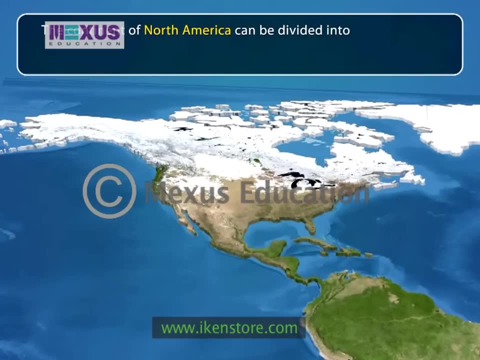 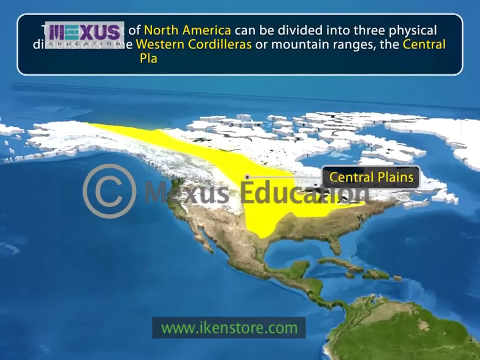 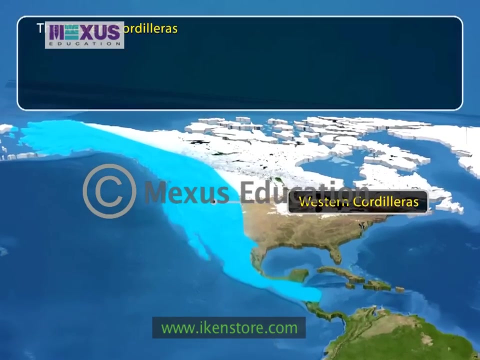 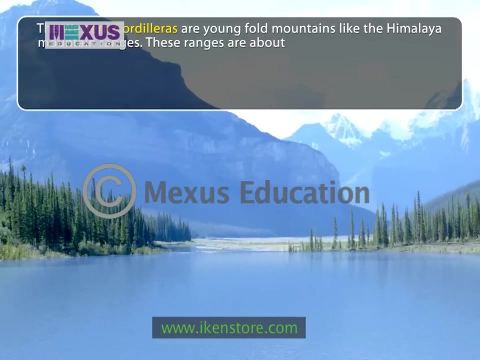 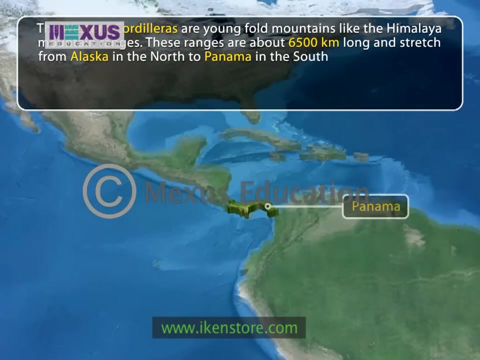 North America physical features. The continent of North America can be divided into three physical dimensions: The Western Cordilleras or mountain ranges, the Central Plains and the Eastern Highlands. The Western Cordilleras are young fold mountains like the Himalaya Mountain Ranges. These ranges are about 6,500 kilometers long and stretch from Alaska in the north to Panama in the south, along the western coast. 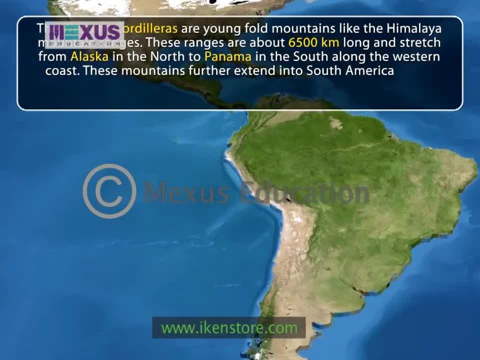 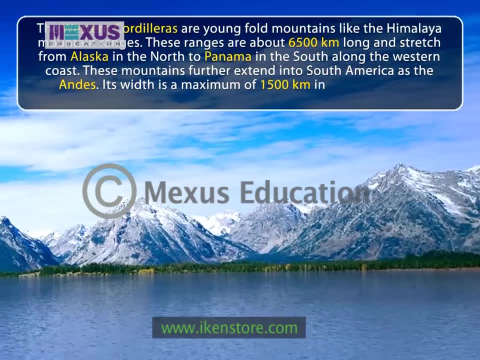 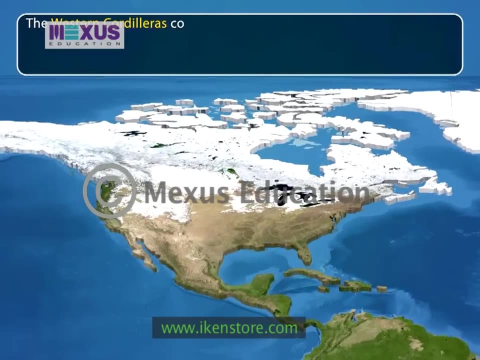 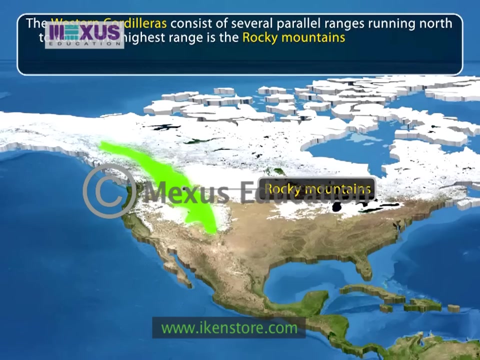 These mountains further extend into South America as the Andes. Its width is a maximum of 1,500 kilometers In the middle and decreases to the north and south. The Western Cordilleras consist of several parallel ranges running north to south. The highest range is the Rocky Mountains, which form the easternmost range. 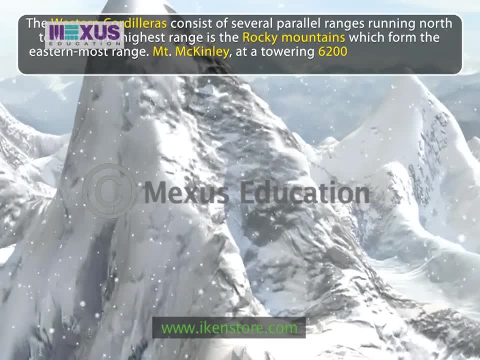 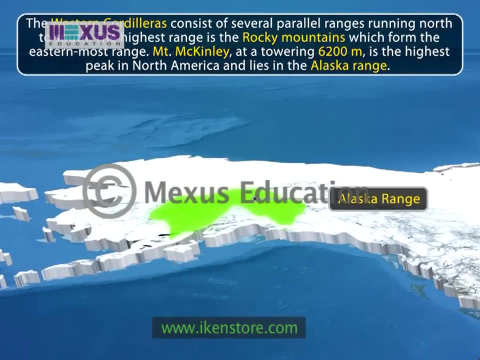 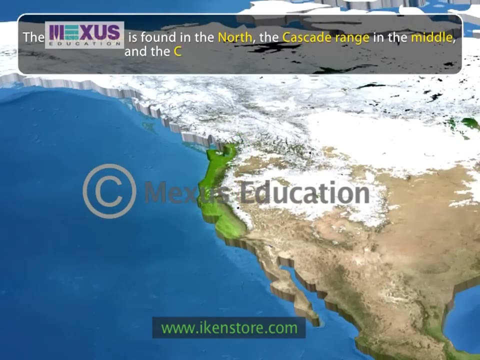 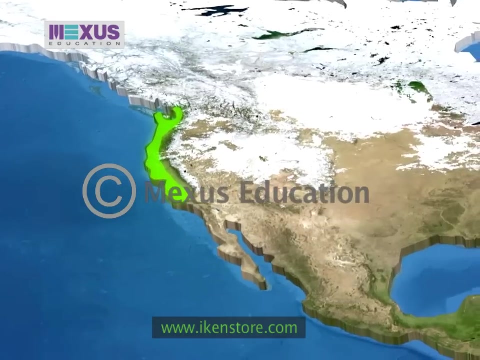 Mount McKinley, at a towering 6,200 meters, is the highest peak in North America. Mount McKinley, at a towering 6,200 meters, is the highest peak in North America. The Alaska Range is found in the north, the Cascade Range in the middle and the Coastal Range along the coast. The Coastal Range in particular rises steeply from the coast. 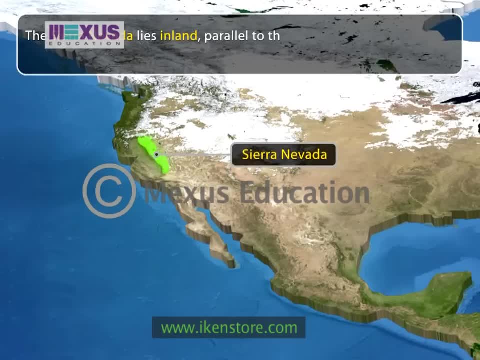 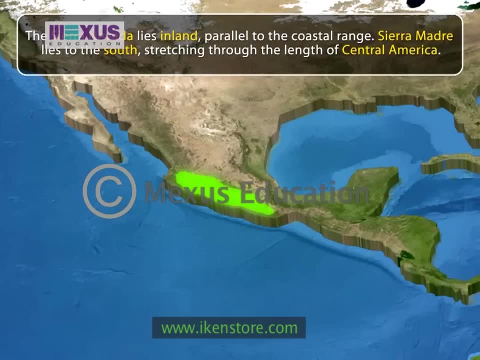